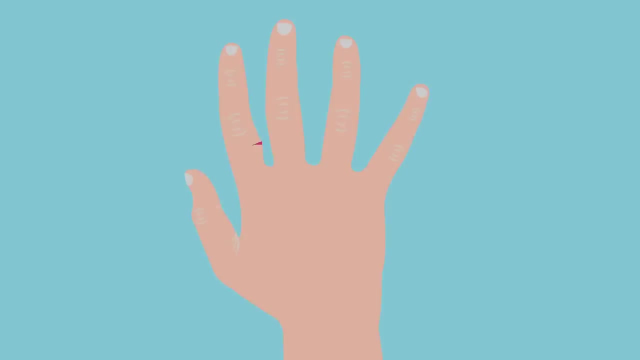 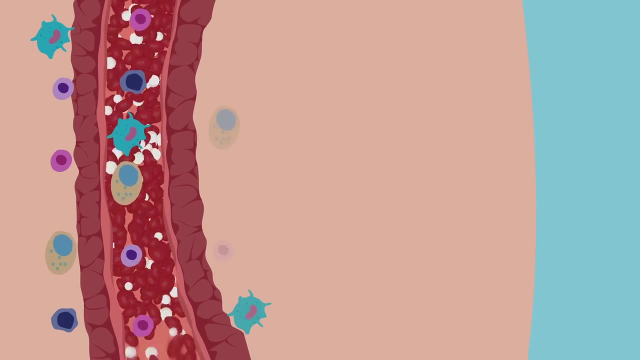 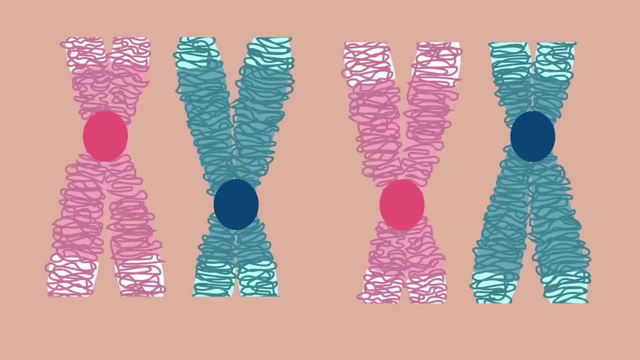 cellular and molecular levels. For example, healthy cells are damaged over time when our immune systems shift from reacting to short-term problems like injuries and infections to gradually producing chronic inflammation throughout the body. Time also gradually shortens the telomeres that act as protective caps for our DNA-containing chromosomes. These and other changes make our 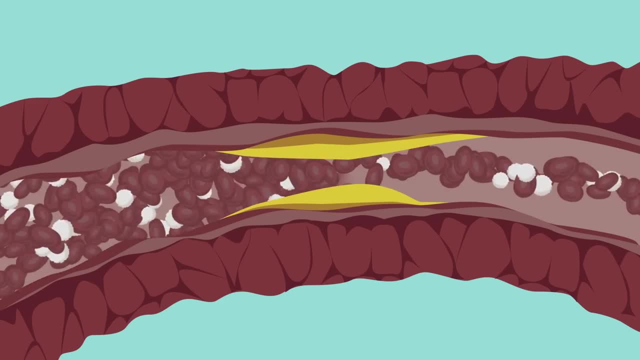 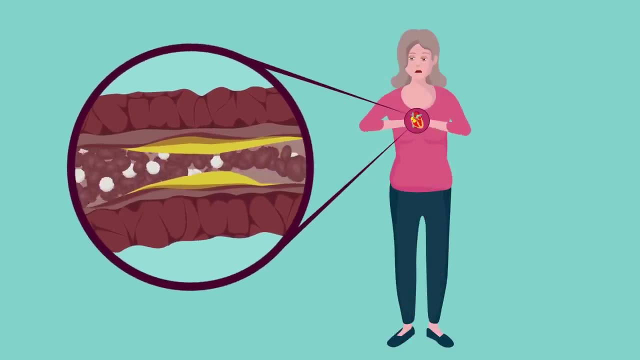 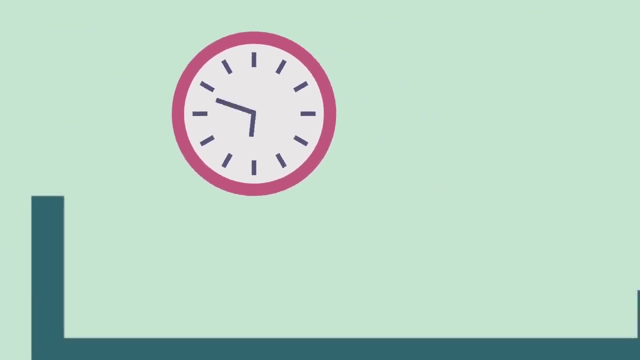 bodies less and less able to deal with stresses from inside and outside of our body. So when damage reaches a critical level, our cells, tissues and organs may no longer perform normally and our health starts to decline. The changes associated with aging start to happen on some level. at day one We begin. 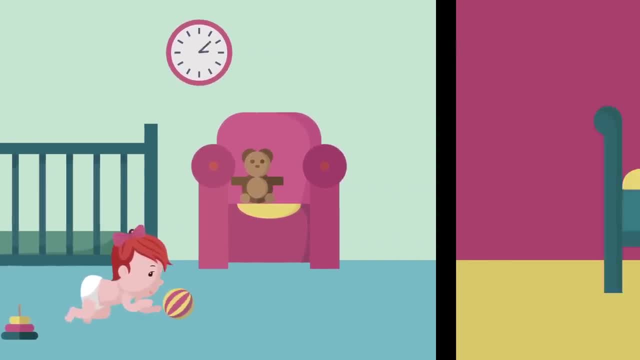 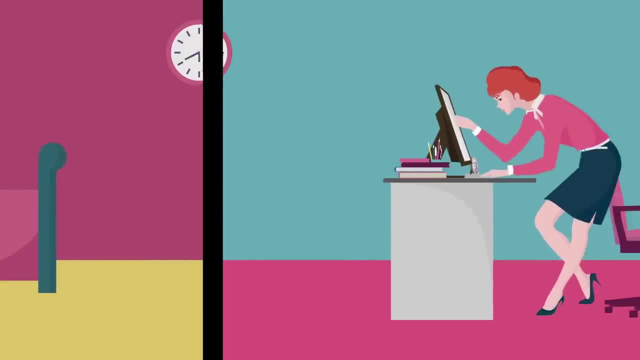 to experience their effects early in life. For example, we lose the ability to hear certain high-frequency sounds as teenagers. Our cognition and memory slowly decline after they peak in our mid-20s. The strength of our bones starts to decrease in our 30s. Female fertility. 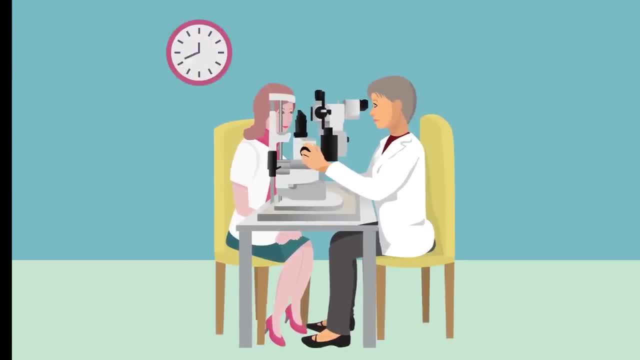 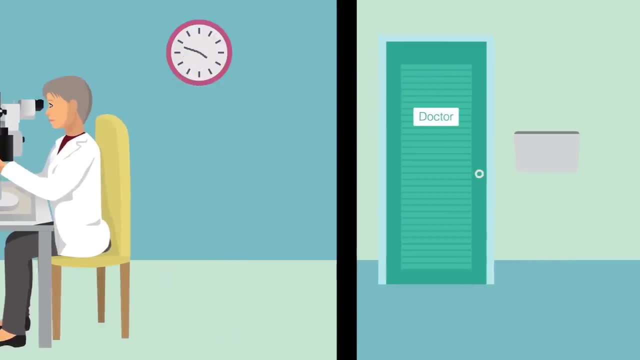 sharply declines after 35.. Age-related nearsightedness begins in our mid-40s, And our hair starts to gray and thin as early as our 30s. After the age of 50, the changes of aging become increasingly noticeable, And because 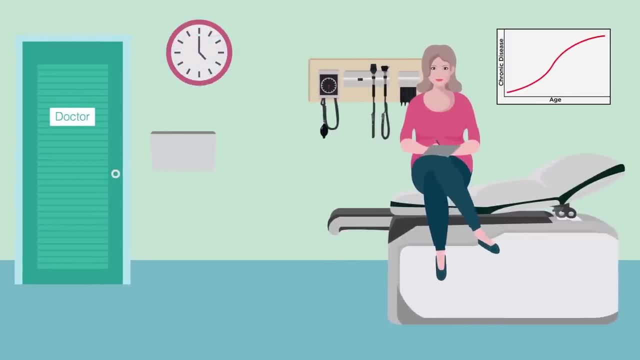 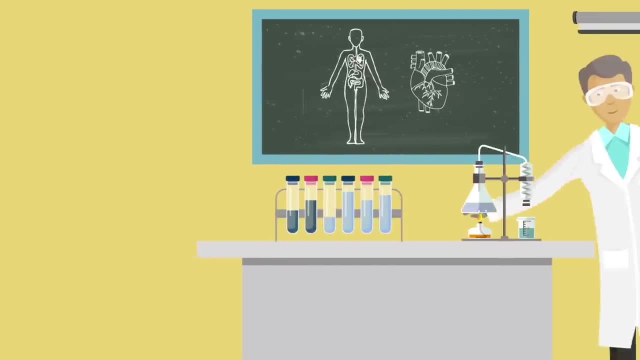 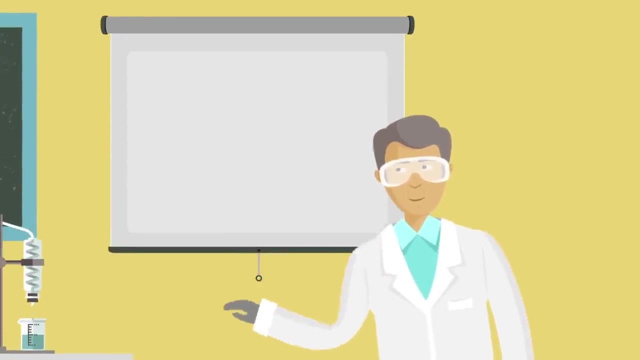 aging is the biggest risk factor for most of the diseases that affect us as adults. the older we get, the higher our risk of chronic disease becomes. While scientists have not yet found a way to stop these processes of aging, they are learning more and more about how to maintain health throughout our lives. Some aspects: 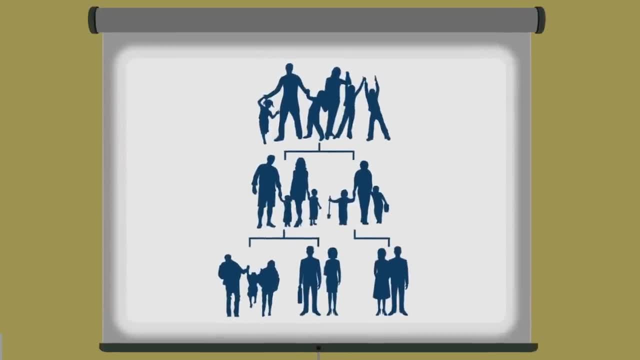 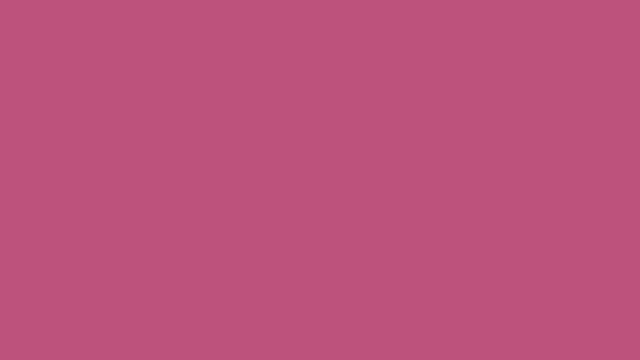 of aging are out of our control, like our genetics and our family history, but we can educate ourselves about moderate risk factors and do our best to reduce them through healthy lifestyle and diet choices. Most of us can be healthy and active well into our later years if we take care of ourselves. 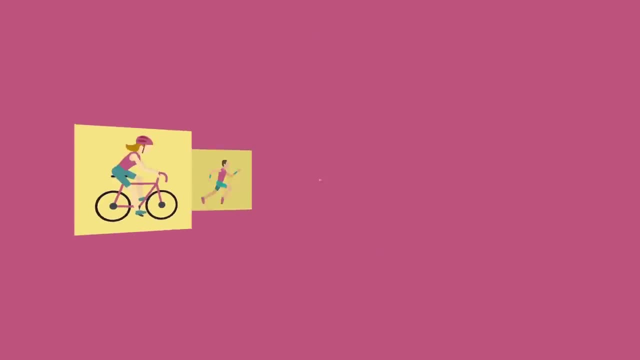 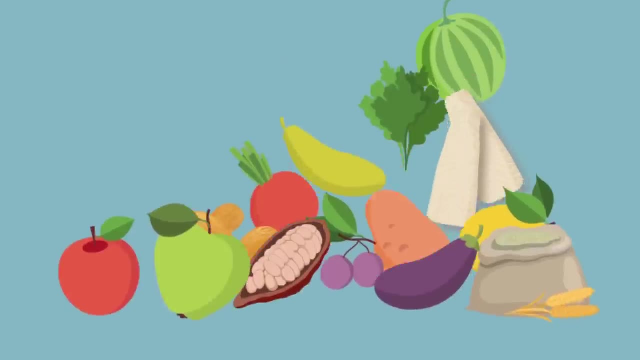 It's no surprise that regular physical activity can help maintain a healthy weight, improve moods and sleep habits and boost overall health. And it's clear that a well-balanced diet full of nutritious foods is critical to good health. But when it comes to understanding,